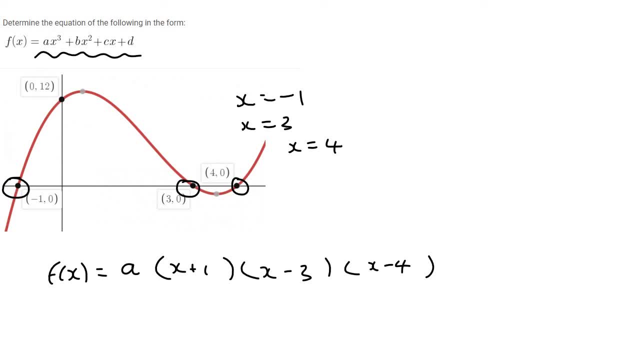 equal to f of x, but then always remember that there should be this random little a in the front. Always remember that when you are asked to find the equation of a graph, Then when you have to find a, you substitute in a random point that you haven't used yet, and that would be this one. 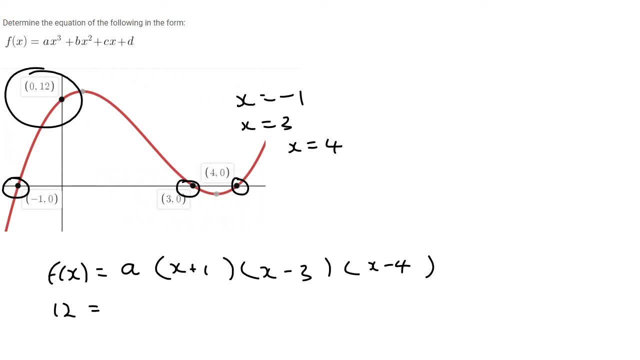 for example. So you could put the 12 in the y's place, x in the zero- I mean zero in the x's place. Then this, these three brackets: just type it all in on your calculator. It's 1 times by minus, 3 times by minus 4.. That's just going to give you 12,. 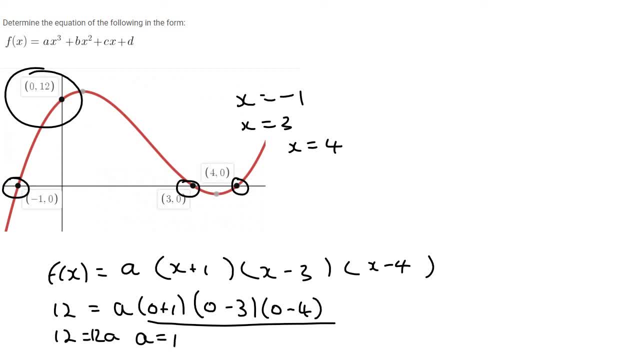 and so we're going to actually end up having 12a, and so a is equal to 1.. So if you did this by yourself and you got a or you left out the a, but you still ended up getting the same answer, 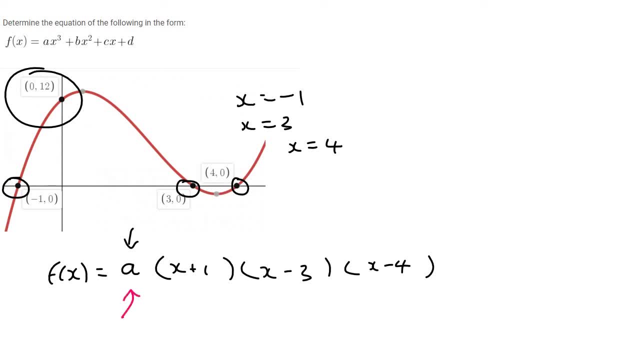 at the end, that's because you were lucky, because a was equal to 1.. But in a test they are still going to mark you down because you haven't done it properly. Okay, so we know that a is 1,. 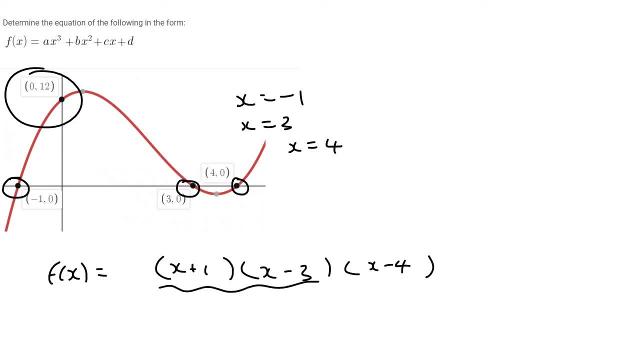 so we don't actually need to put it there, because a 1 doesn't do anything. Now, what we do is we just multiply these brackets together, and so I'm going to multiply the first two brackets together, and that would give you x squared minus 2x minus 3.. Eventually, you might do it the longer way. 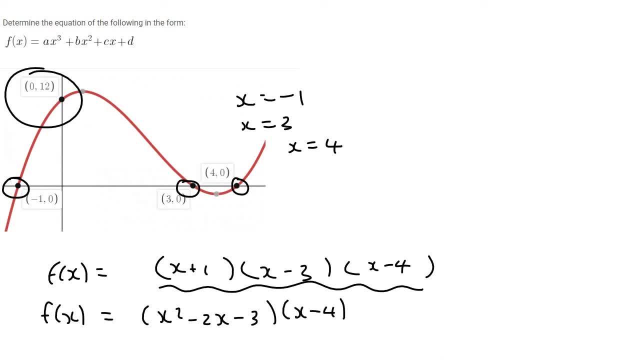 that's absolutely fine, and then we're still left with x minus 4.. Now I like to put the x minus 4 in the front. It's always nice to have the smaller bracket, and then the bigger bracket makes it a bit easier. 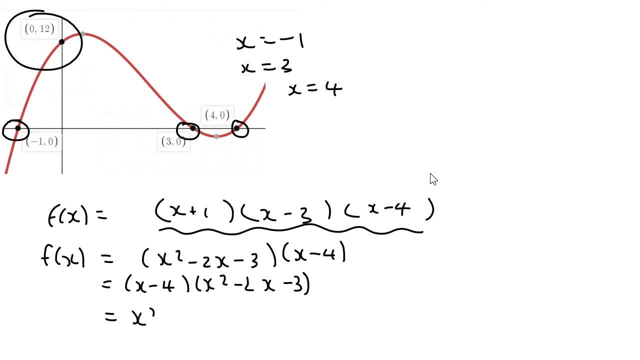 Okay, and you guys know how to multiply this all out, but I'm just going to do it: 2x squared minus 3x, minus 4x squared plus 8x plus 12.. We then put the like terms together, that's x3. 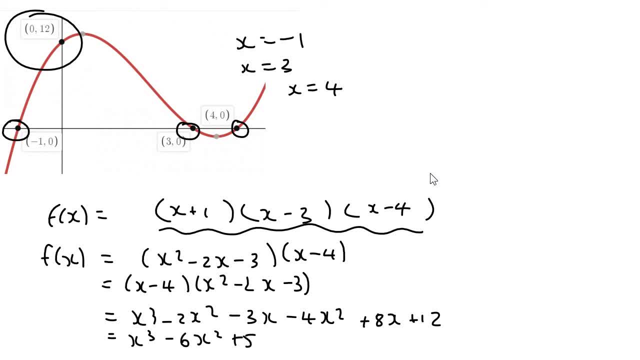 minus 6x, squared plus 5x plus 12.. And so f of x is equal to that. So the main thing I want you to take away from this lesson is that when your x intercepts are given, turn them into brackets.